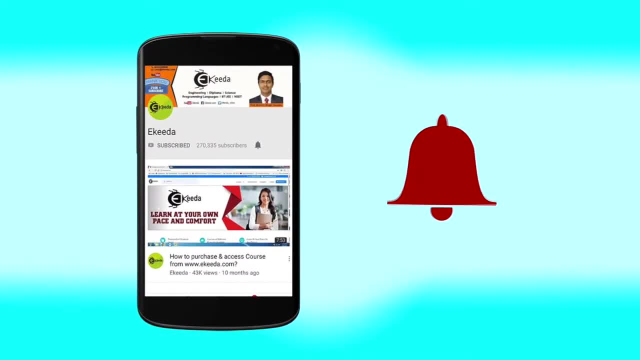 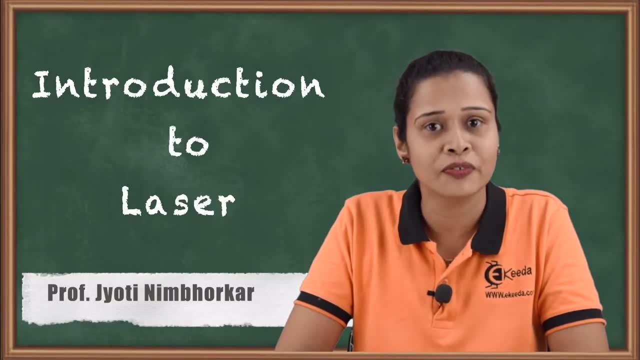 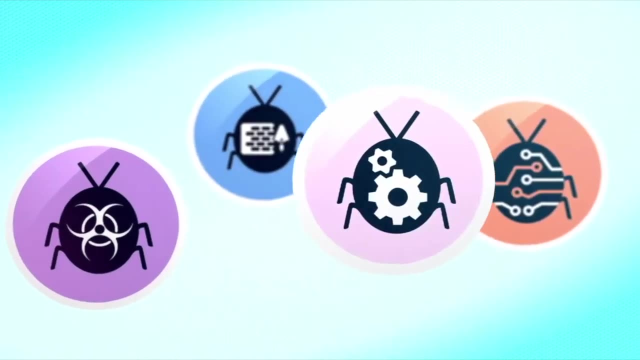 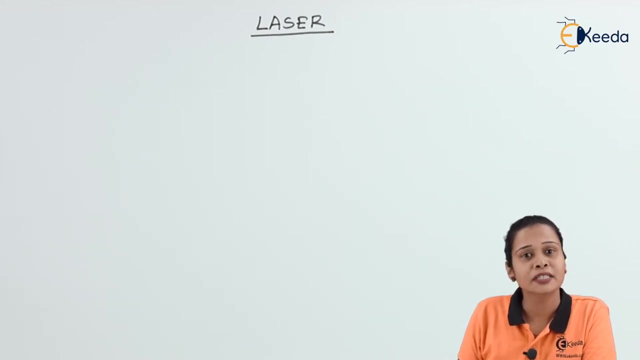 Click the bell icon to get latest videos from eKIDA. Hello friends, today we will see introduction to laser and what is the difference between ordinary source of light and laser. Now, before start laser, we should know what is the monochromatic source of light and what. 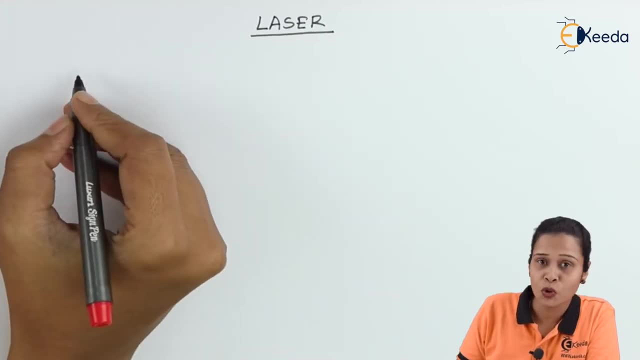 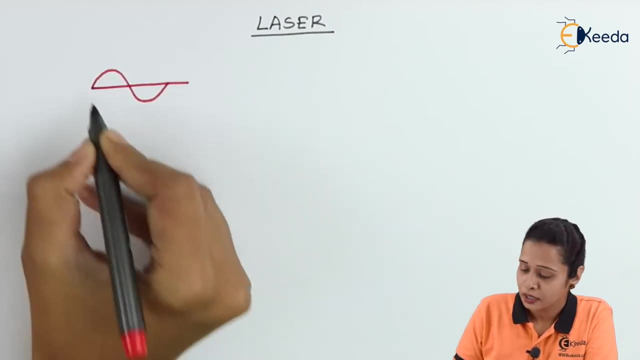 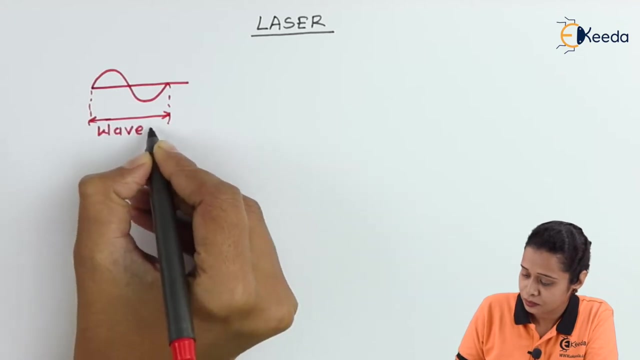 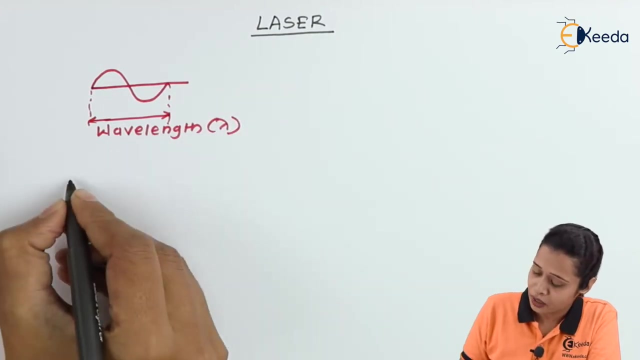 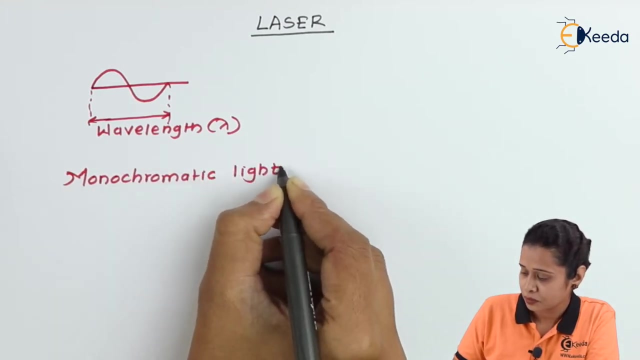 is meant by coherent source of light. So we will see monochromatic source of light, Suppose we are considering wave. So this distance is called as wavelength, which is mean wavelength is significant length just below the wavelength of a wave. 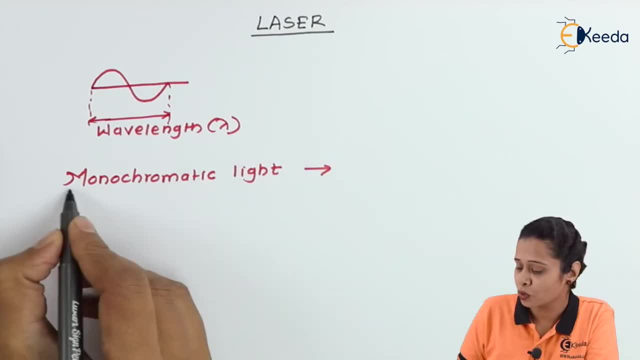 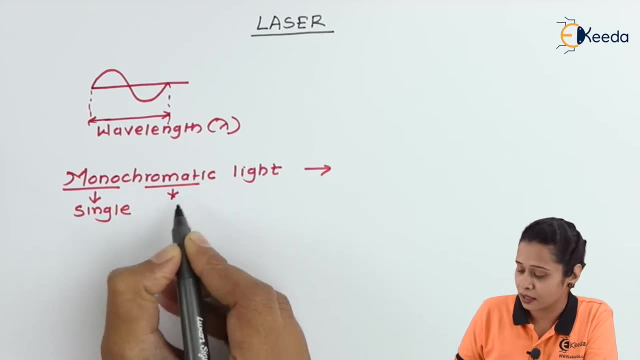 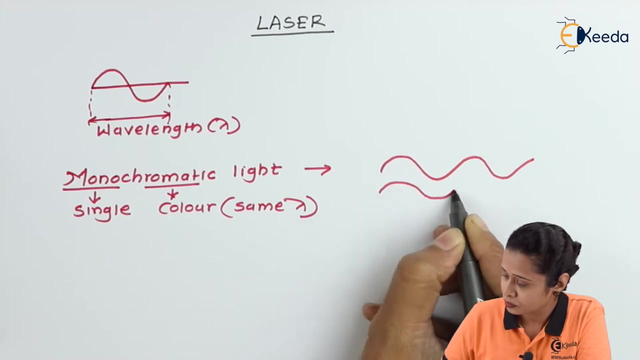 Means lambda, should be same Mono. mono means single, Chromatic means colour, Single colour means same lambda. So this type of light rays called as monochromatic light, or the source called as monochromatic source of light light. So suppose we have Now in this three diagrams three waves. we have same wavelength. 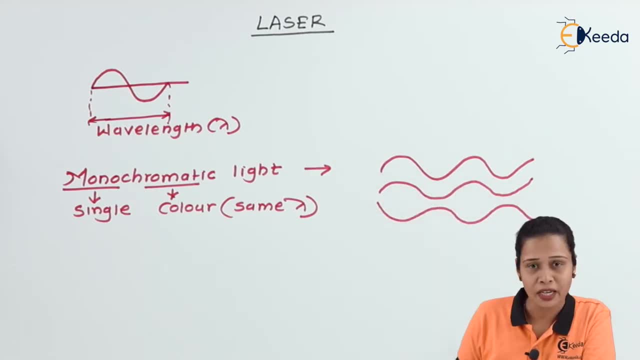 The wavelength of light is same. That's why we can say this is monochromatic source of light. But we can see the phase is not same. So we have a second term that is coherent. Coherent means if the waves are traveling with same phase or no phase difference. 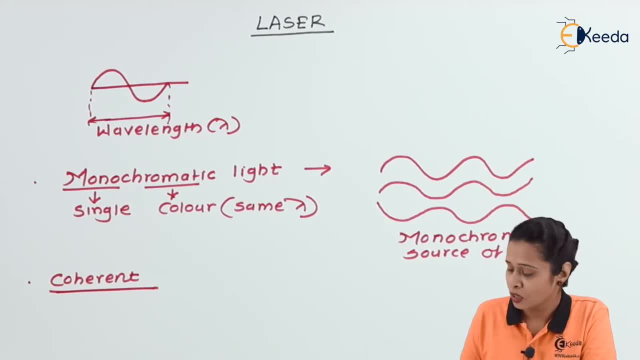 then we can say: this is a coherent source of light. So for coherency we should require a monochromatic source first. So if we have a monochromatic source- means lambda is same- and we have a monochromatic source, then we can say: this is a coherent source of light. 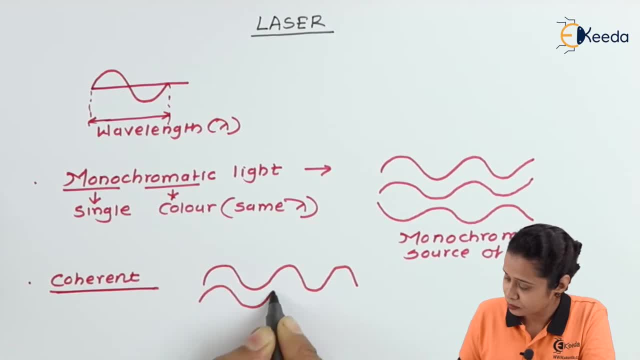 And they are traveling with the same phase. Then this source of light is called as monochromatic and coherent source of light. So coherent means same phase or no phase difference. Let us see the second diagram, Other source of light here Now, first source we have that is consist of three waves. 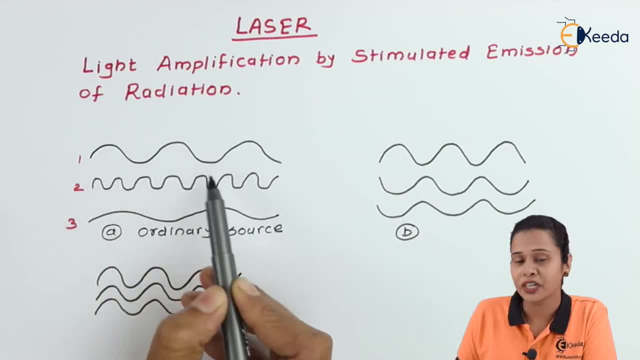 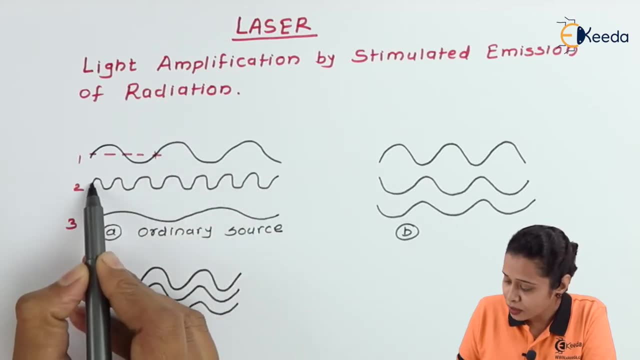 If you observe this, three wave, all three waves having different wavelength. This is the wavelength of first wave, first source, This will be the wavelength of second source And here we have a wavelength of third source. So here the wavelength is a different, as well as 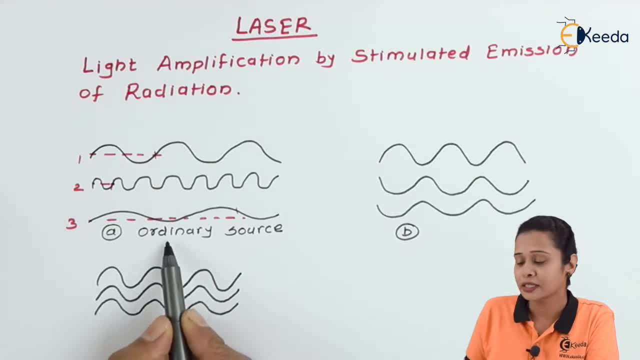 this second source. So in this second diagram the wavelength is a different, as well as the wavelength is a different, our phase is also not same Means we can say: this is ordinary source of light. If we want the example of ordinary source, we can say: the light coming. 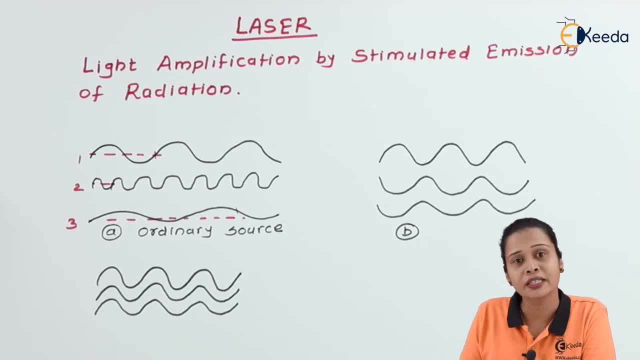 from the candle or light coming from the sun. It's a ordinary source of light. Then we will see the second diagram. In this second diagram, if we observe the wavelength of all the waves are same. when there is the same wavelength we can say it's a monochromatic light. but if you observe the phase, 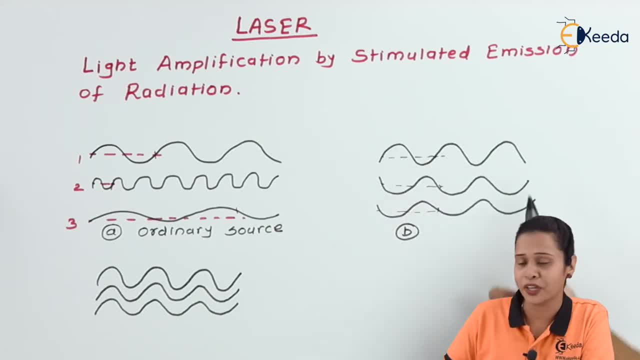 there is a phase difference between these three waves means this is a monochromatic but incoherent source of light. now look at the third diagram. in this third diagram we have again three rays. all three are traveling with the same phase, as well as their wavelength is also same. 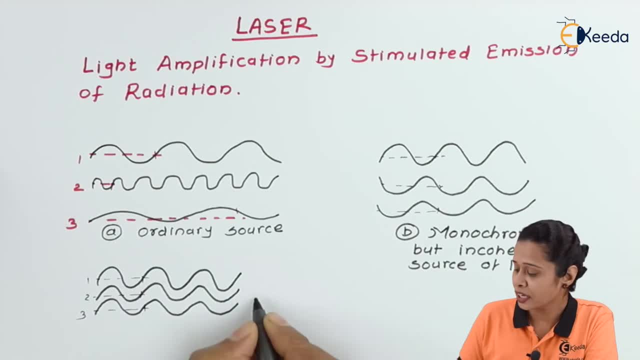 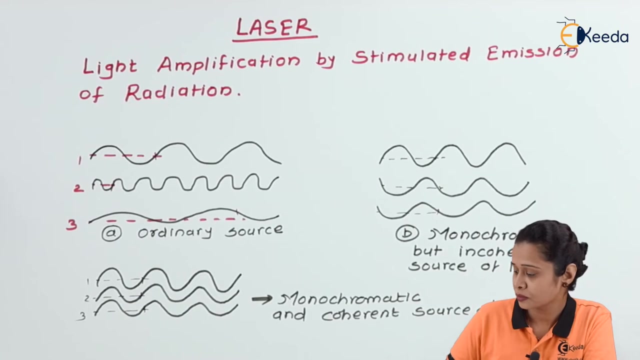 means we can say when there is a wavelength, same means it's a monochromatic, and when there is a no phase difference, all traveling with the same phase means coherent. so this is monochromatic, monochromatic and monochromatic and coherent. source of light. 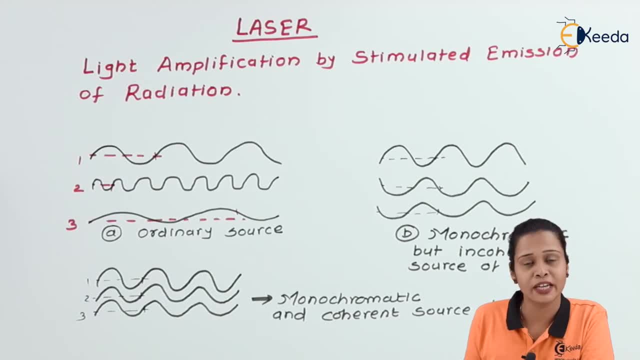 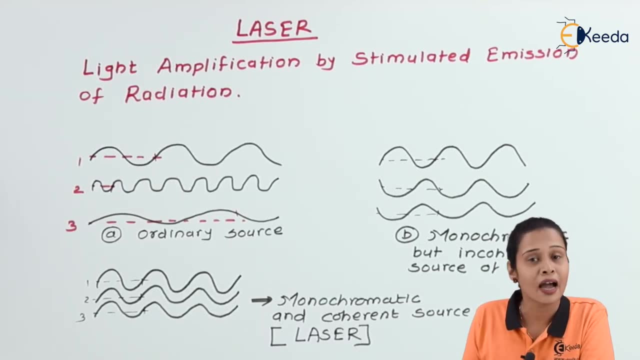 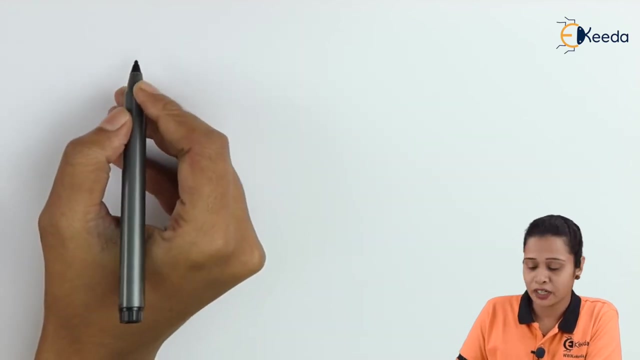 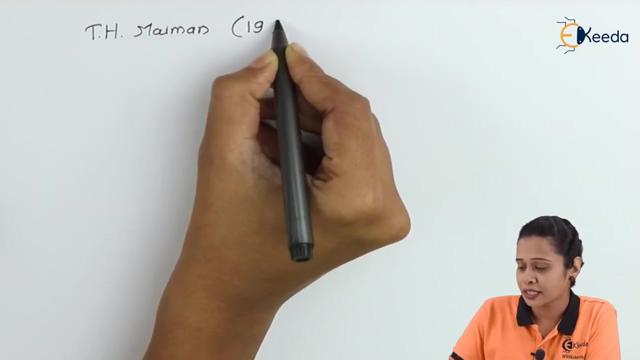 and example of monochromatic and coherent source of light is a laser means. laser is highly monochromatic and highly coherent source of light. so let us see what is the long form of laser. laser is light amplification by stimulated emission of radiation. Laser discovered by TH Maimon in 1960. 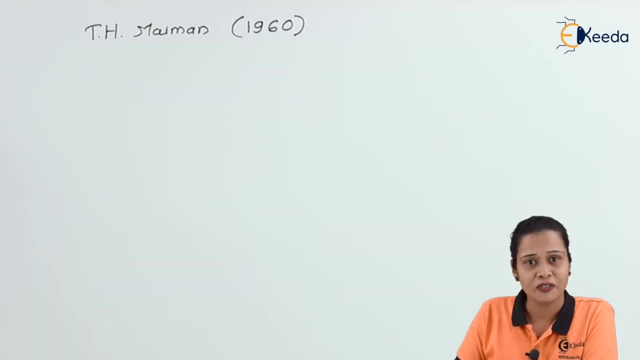 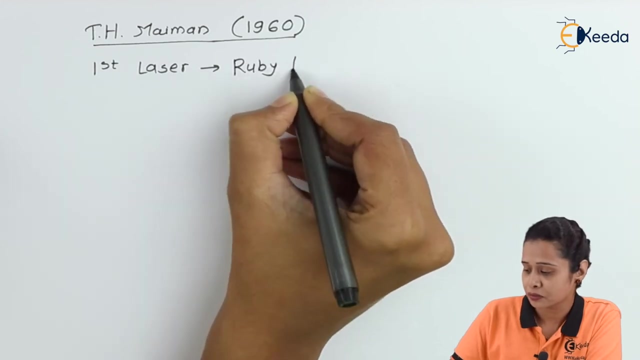 after the discovery of stimulated emission by scientist Einstein and stimulated emission discovered in 1917.. After that, after few years, there is a discovery of laser by TH Maimon And the first discovered laser is ruby laser. It was three-level laser system. 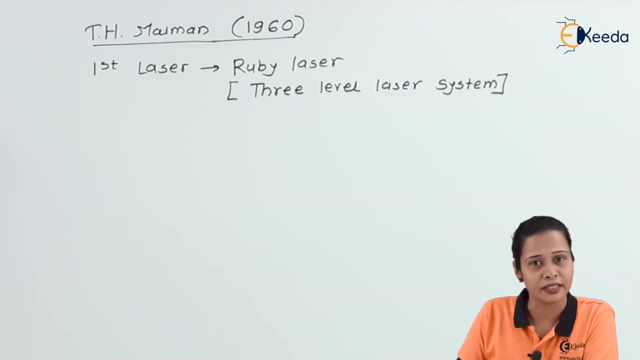 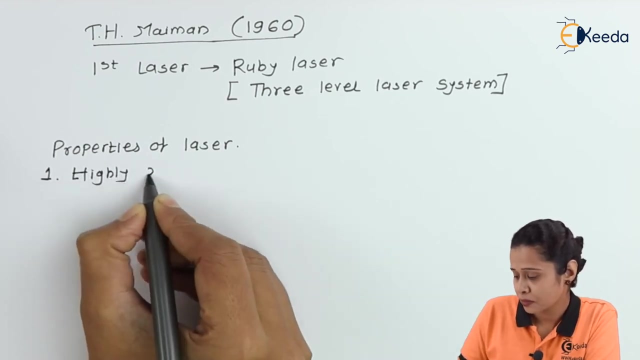 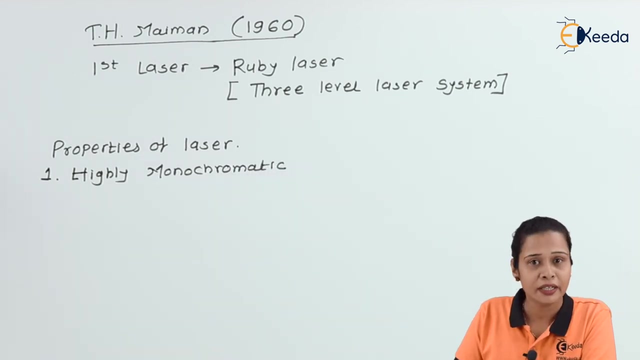 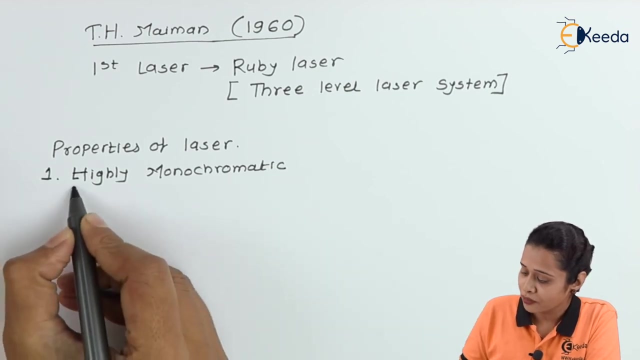 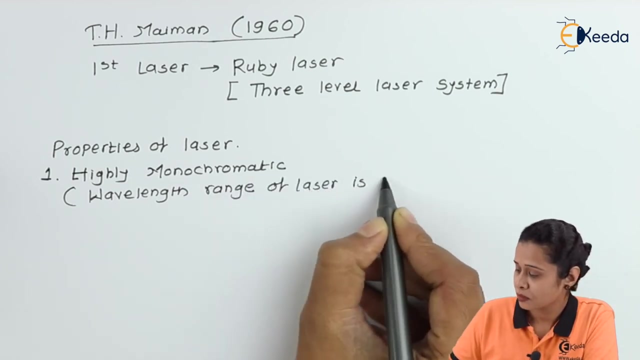 Now we will see what are the properties of laser. Laser is highly monochromatic Means, there is only one wavelength. But the wavelength range of laser is from X-ray to the microwave region, So wavelength range has a completely different length. comparison with interacting with touch measuring of radar letters. 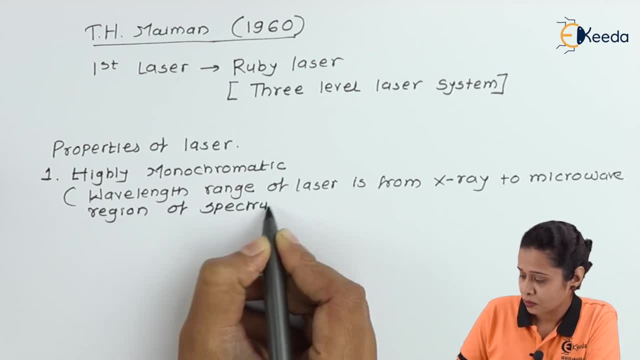 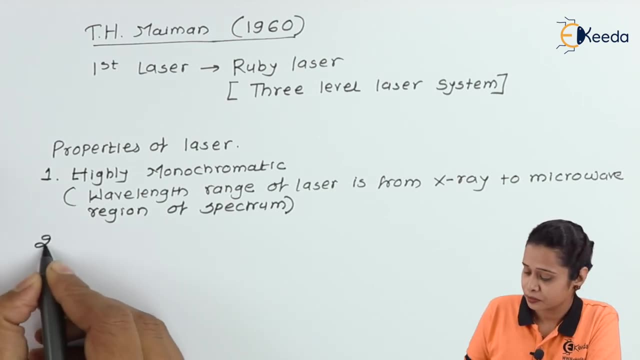 Laser is highly monochromatic based on its number of rays. Then way laser sûrces. the existing ages didn't apply again. But if you can 영화 to theiąg HSL, Then you can talk. Laser is highly Mil hopeful on Earth. 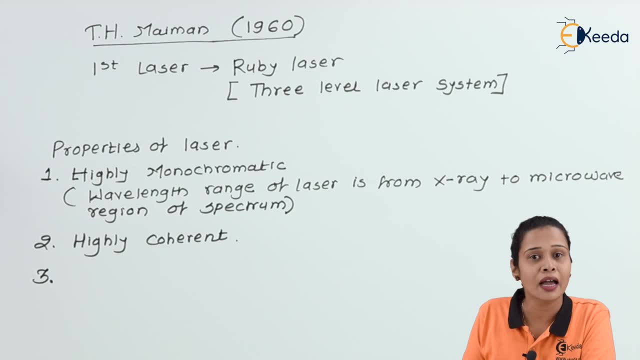 visibility quality. it is highly directional means the divergence is very small. that's why it travel a very long distance and that's why there are huge number of application, as it is highly directional. next is size of laser. the size of laser is varies from one tenth of the diameter of human hair.